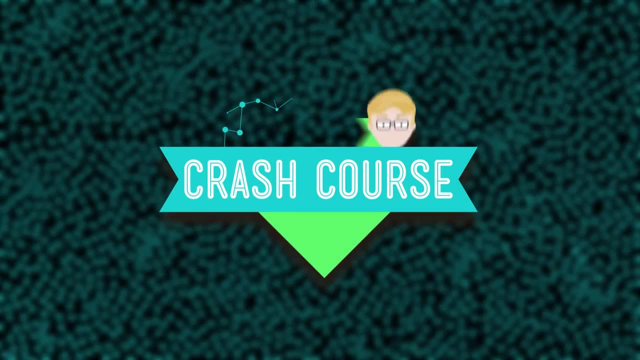 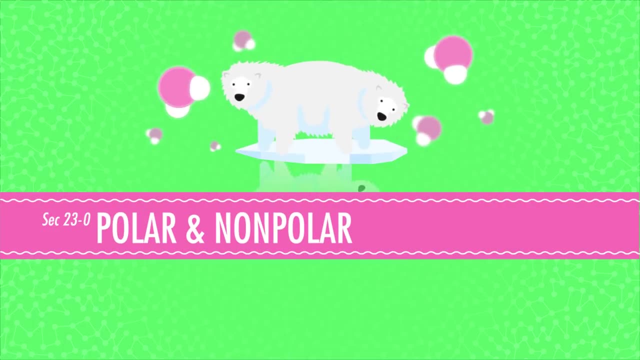 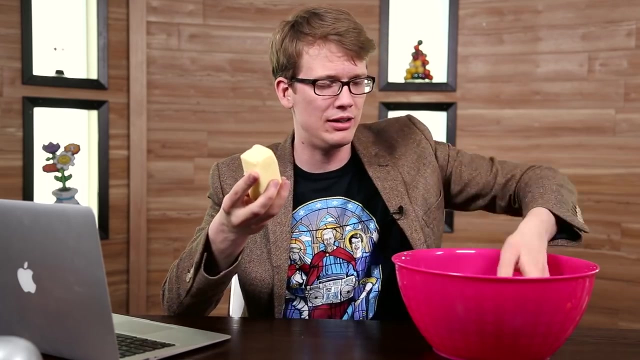 but polar, in my humble opinion, is where it's at All. right Now, here are two very different types of chemicals. Right here I have a stick of butter, and then in this bowl that's just normal water. So I'm just going to go ahead and squeeze this butter which, if you're wondering, is: 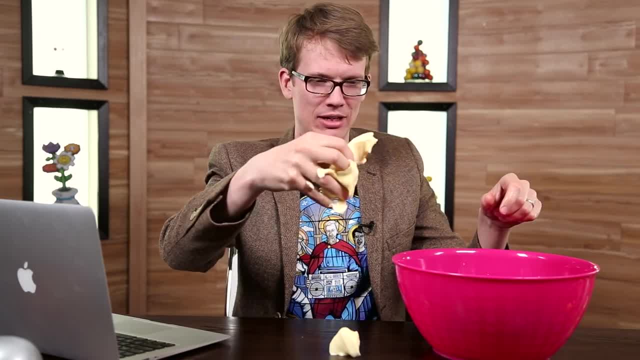 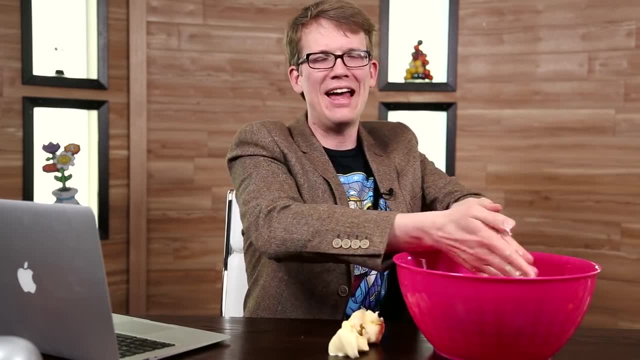 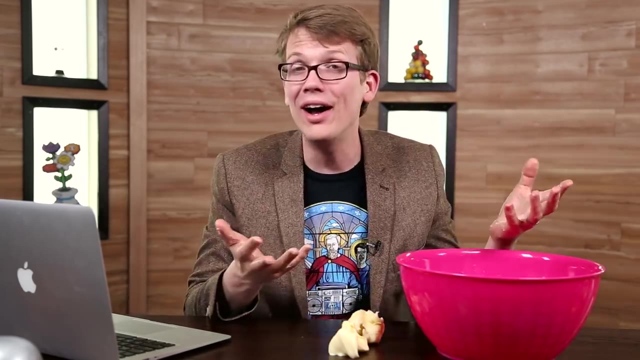 both a terrible and wonderful feeling, And then I'm going to just drop that. Now I'm going to attempt to wash that butter off my hand, but that is just not hap- that's just. it's not going anywhere ever, Ever. That's, it's just beating up on me. Why? Because water. 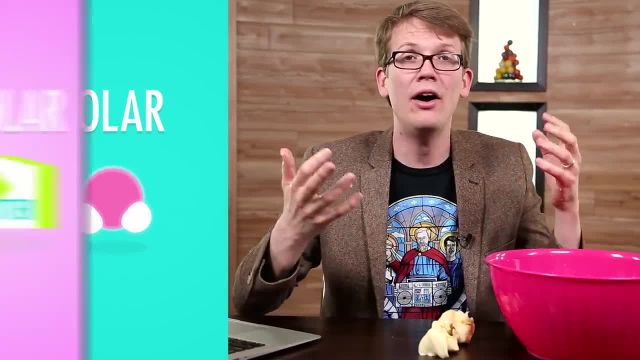 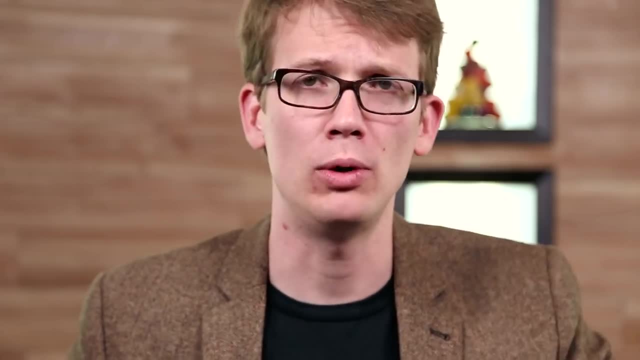 is a polar molecule and the various chemicals that make up butter are the chemicals that make up butter are nonpolar, and water wants nothing to do with that Ugh. So what makes a molecule polar? Well, two things. First, asymmetrical electron distribution. 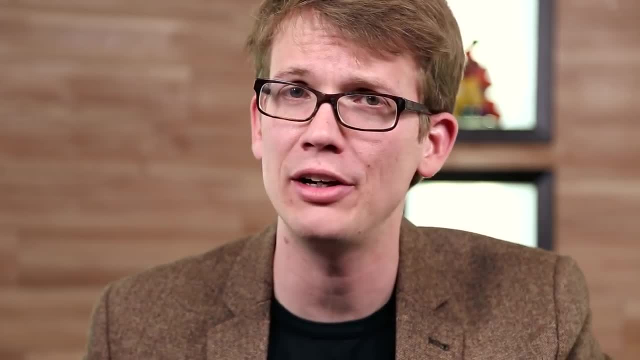 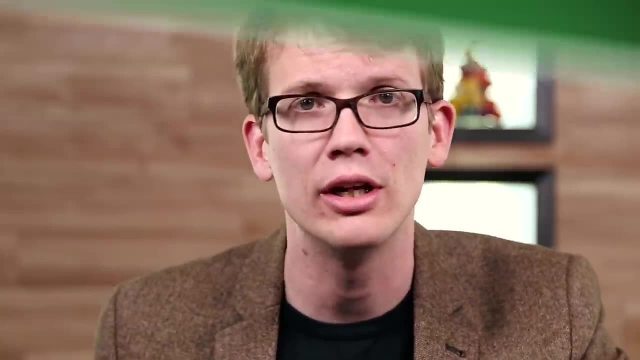 around the molecule. You can't have a polar molecule made up entirely of the same element, because those atoms will all have the same electronegativity and thus the electron distribution would be completely symmetrical. Electronegativity is usually thought of as how much an element. 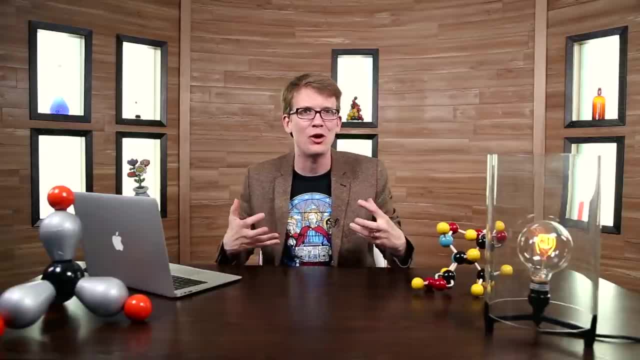 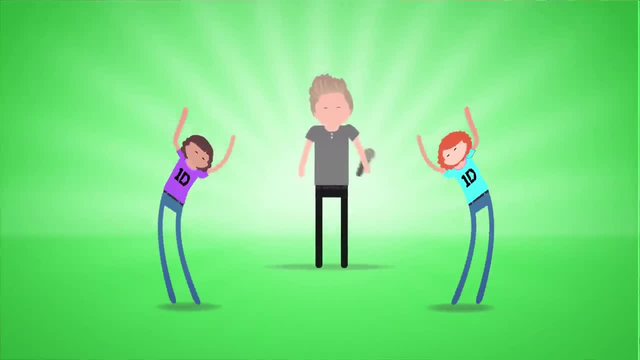 wants electrons around it, but I think it's more about how much electrons want to be near that element. If electrons were 13-year-old girls, fluorine would be Niall Horan. They'll do anything just to be near it. Why? Some simple periodic trends: Electronegativity. 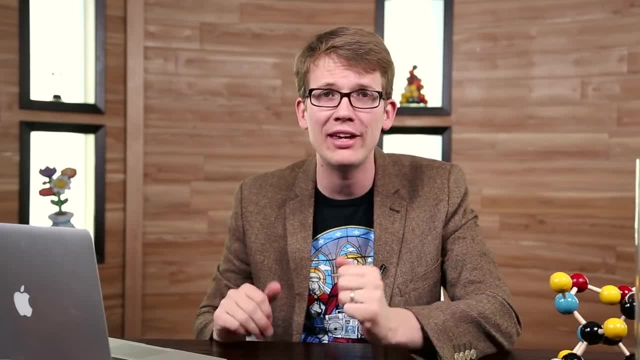 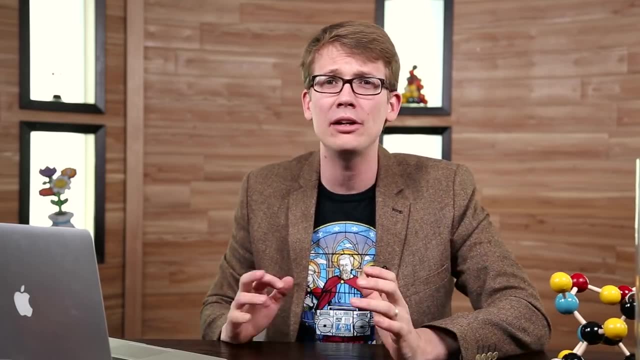 increases from left to right because there are more protons in the atoms, and more protons means more boys in the band. Meanwhile, it decreases as you move from top to bottom because, as the crowd of electrons gets bigger, they start to shield each other from the effects. 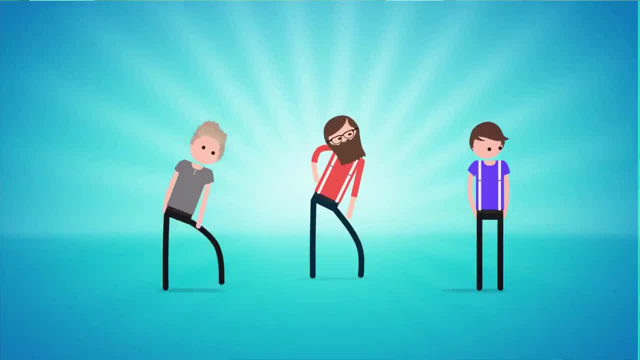 of the protons. What I'm trying to say is that electrons are hipsters. If a bunch of other electrons are into that thing, they're less interested. Now, there are a number of other factors here, but just like the relationship between tweens. 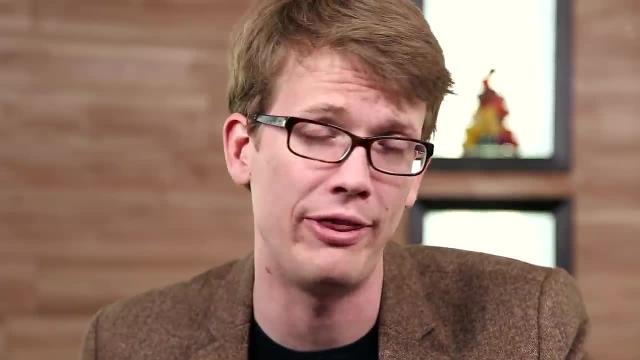 and their latest boy band fixation. it's complicated and weird and you probably don't want to think too much about it, But in this nice little map you can see that the trend is pretty clear. The upper right is where all the superstars of electro-fame are: Oxygen. 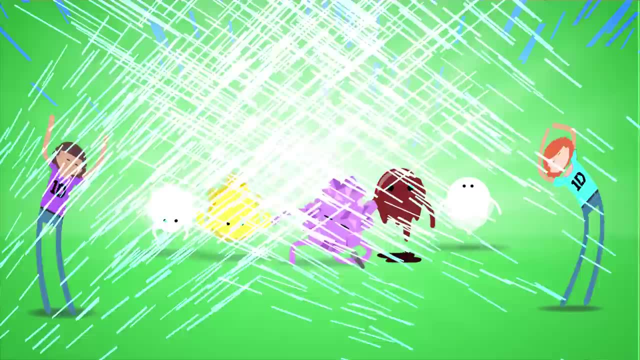 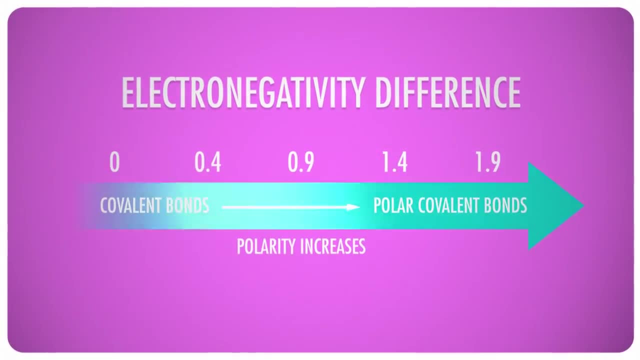 nitrogen, fluorine, chlorine and bromine are basically the one direction of the periodic table. So for polarity to occur in a molecule you have to have two different elements at a minimum, and the difference between their electronegativities has to be 0.5 or greater. 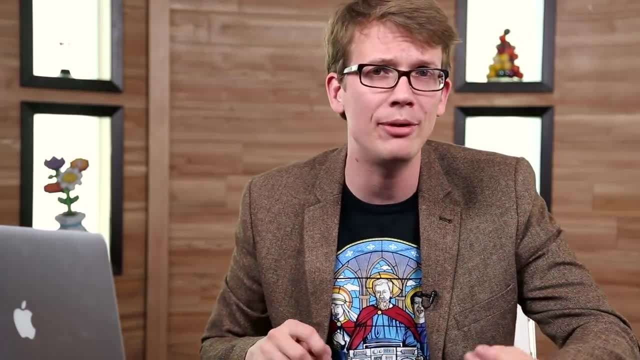 If that's the case, the output will be 0.5 or greater. If that's the case, the output will be 0.5 or greater. The outer electrons spend enough extra time around the element that's more electronegative. that chemists label the molecule polar. The result is a. 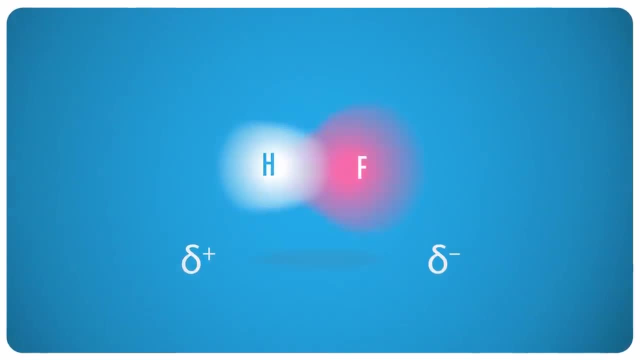 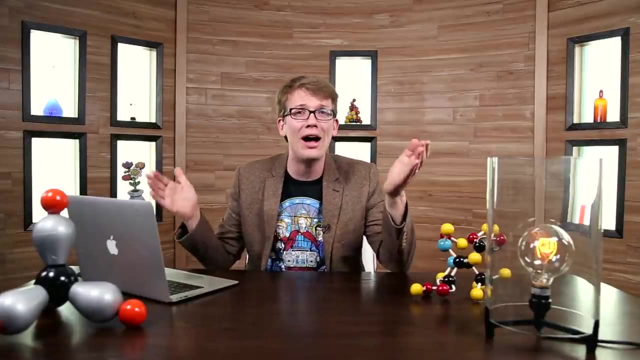 partially negative charge on the more electronegative part of the molecule and a partially positive charge on the less electronegative side. Now, in extreme cases, like if the electronegativity is greater than 1.6, then we end up with two. 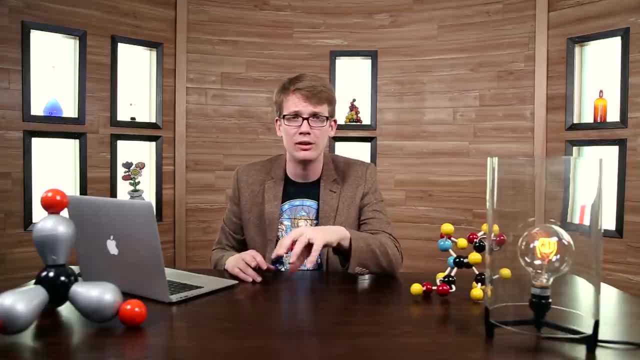 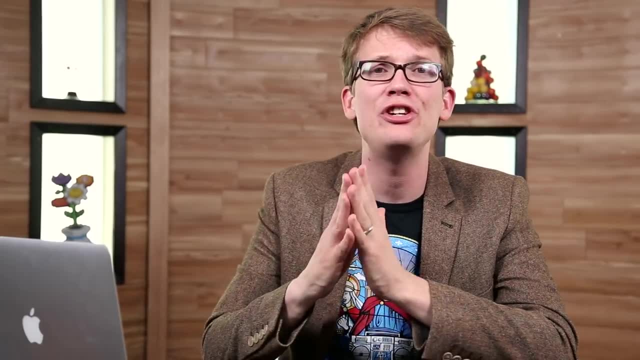 ions in the same molecule. This isn't what we're talking about here. when we talk about polar molecules, We're talking about differences between 0.5 and 1.6.. Another requirement for polarity: you've got to have geometrical asymmetry. CO2 is 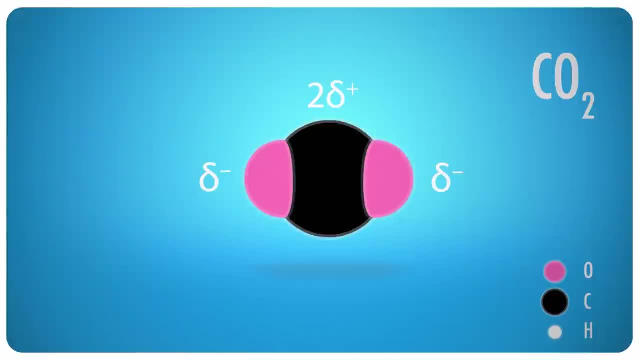 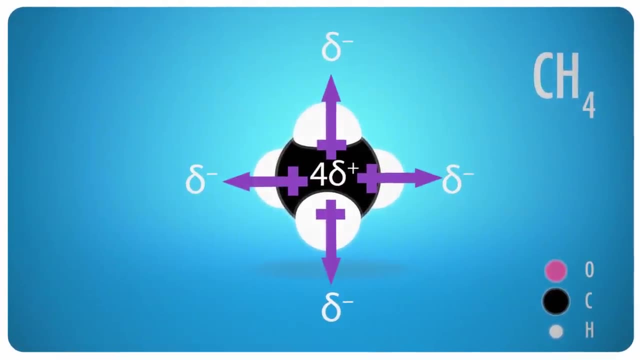 here has the charge asymmetry locked up, but because the molecule is linear in a straight line, it's a kind of symmetrical asymmetry. The same thing goes for CH4, with its tetrahedron of weakly electronegative hydrogens around a more strongly electronegative carbon. 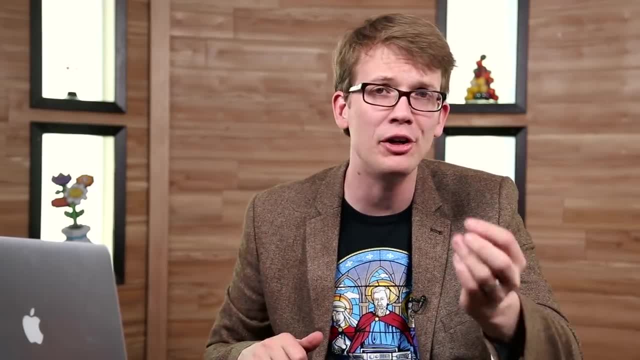 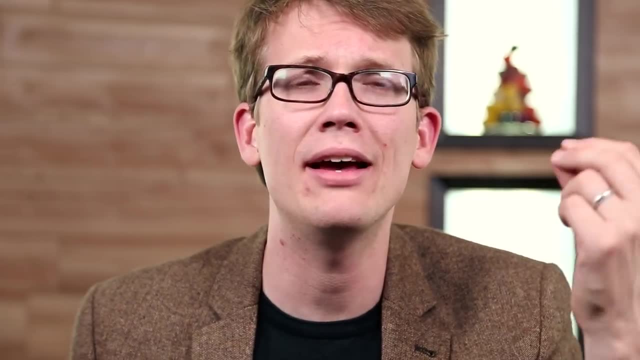 These molecules have polar bonds, but the molecules themselves are not polar because the symmetry of the bonds cancels out the asymmetry of the charges. In order for a molecule to be polar, there has to be a dipole moment, a separation of the charge around the molecule. 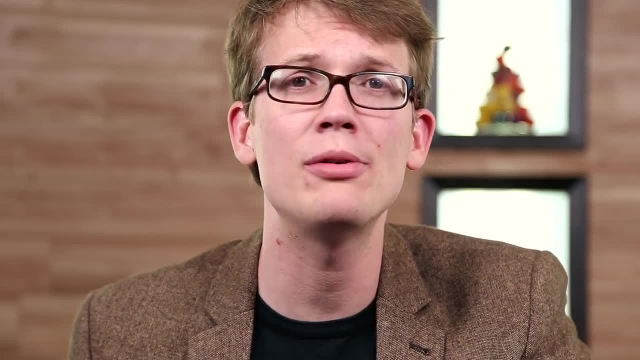 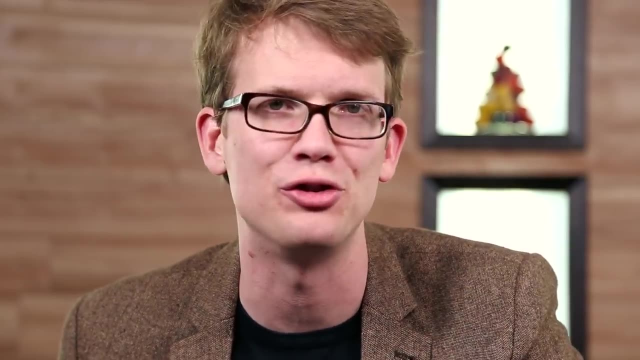 into a more positive area and a more negative area. Lots of molecules are asymmetrical in both electronegativity and geometry. Those are our polar molecules, the asymmetrical beauties of chemistry. Look at them all. They're so quirky and weird. 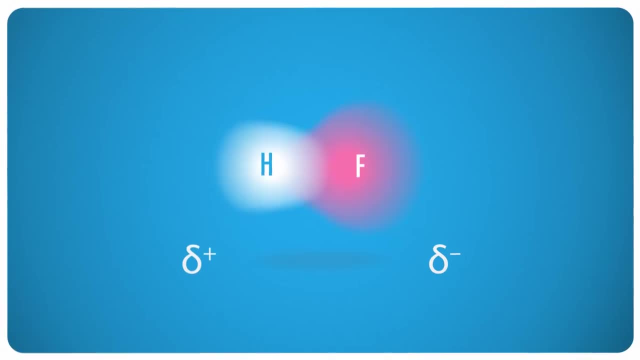 We've also got a system for indicating where their charges are. We draw an arrow with a plus sign at the tail, pointing toward the negative side of the molecule. Little lowercase delta plus or delta minus by the individual atoms signify a partial positive or partial. 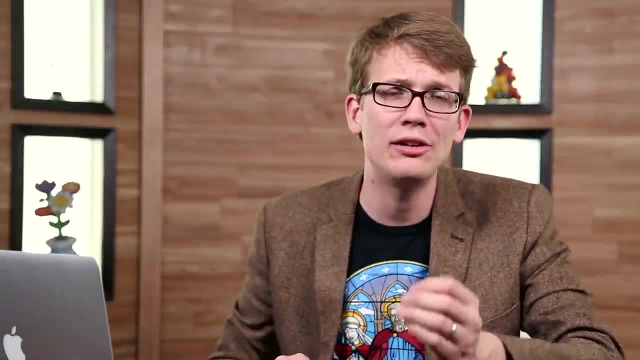 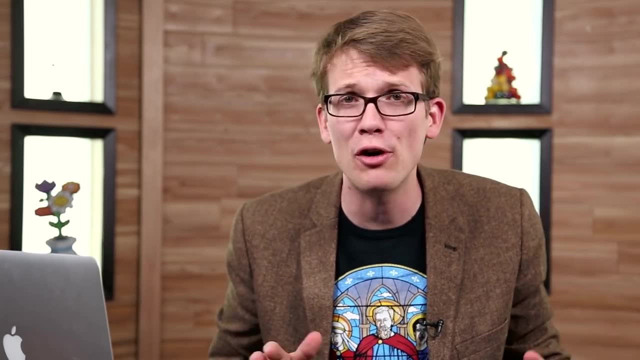 negative charge. These molecules are really good at dissolving solids that are composed of polar or ionic compounds. Ionic solids are basically just polarity taken to the extreme so far that, instead of having a partial positive and partial negative dipole moment, the electrons have 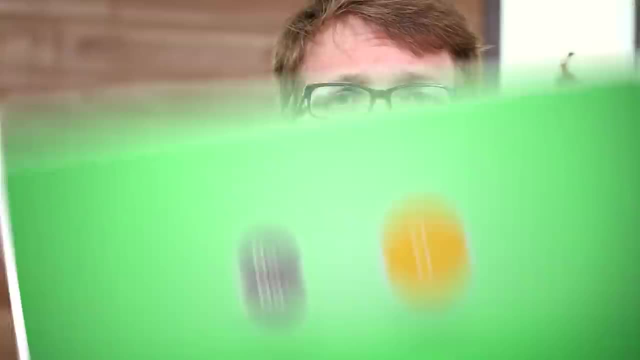 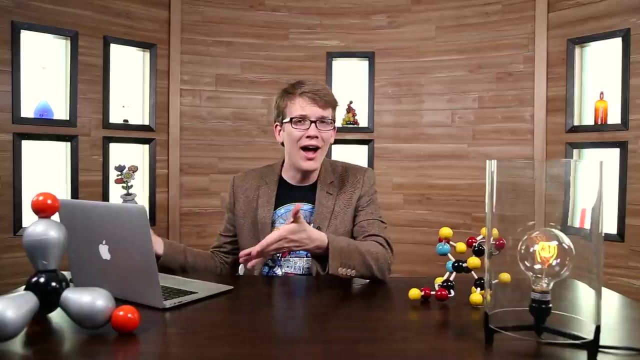 completely transferred, creating two charged ions. Now I assume we've all heard that like dissolves, like, so the easiest way to figure out if a liquid is polar or nonpolar is just to dump it in some water. But the why of this? 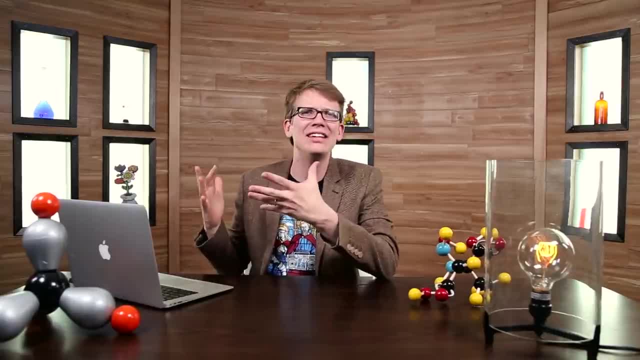 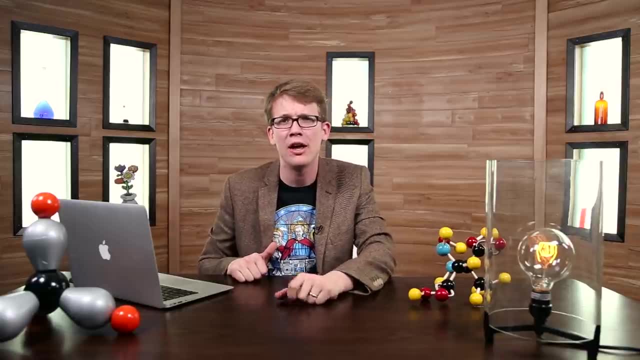 phenomenon is usually just totally glossed over. What's actually happening to those molecules? It's like they're all just bigots, terrified of anything even a little bit different than themselves. But this is chemistry, so there must be some fundamental reason. And if it's, 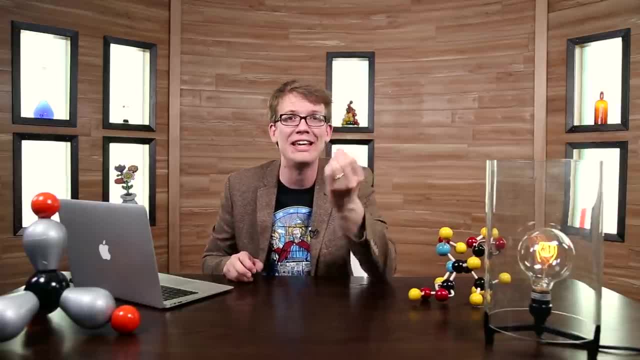 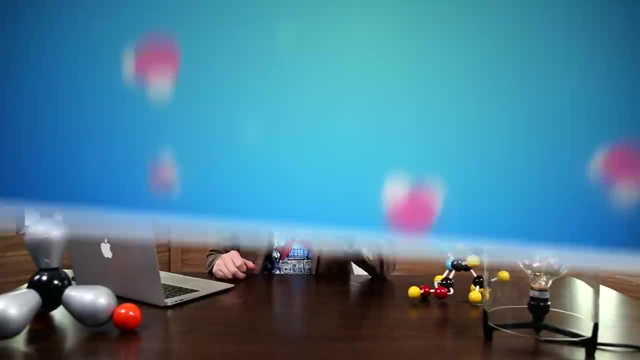 fundamental. it probably has something to do with decreasing the energy of the system- And indeed it does- Those partial positive and partial negative charges of water. They're at their lowest energy state when they're lining up together positive to negative into a kind of liquid. 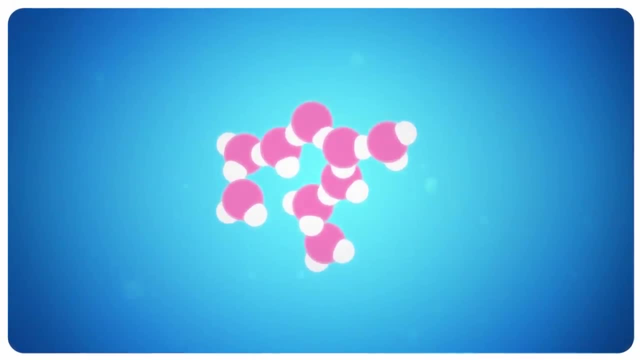 crystal. There's an arrangement there. It flows, of course, but the oxygen sides are always doing their best to orbit around it, And that's why it's so important that we have a system like this. We have a system like this. We have a system like this We have. 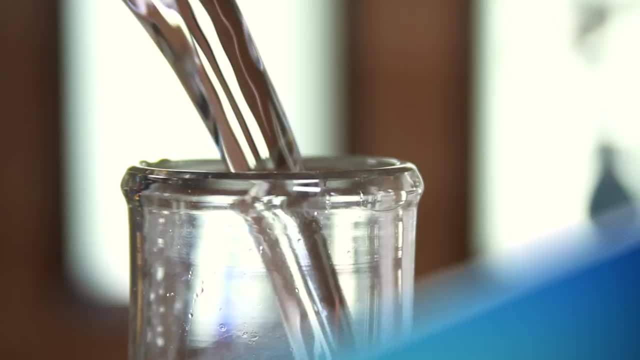 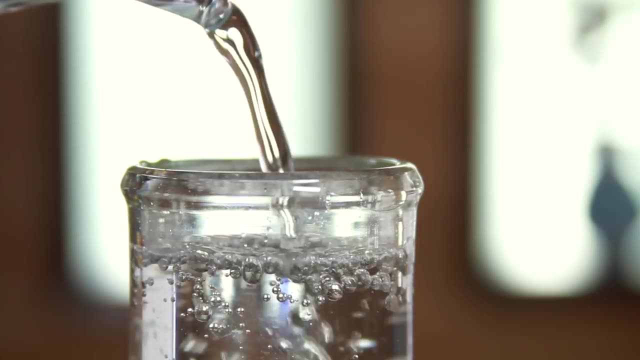 NOTHING but apple parts that are inside the surface that can orient themselves toward the hydrogen sides of other molecules. You can even see the effects of that attraction as the surface tension that allows me to pour more than 100 milliliters of water into a 100-mill container. The strength of that surface. 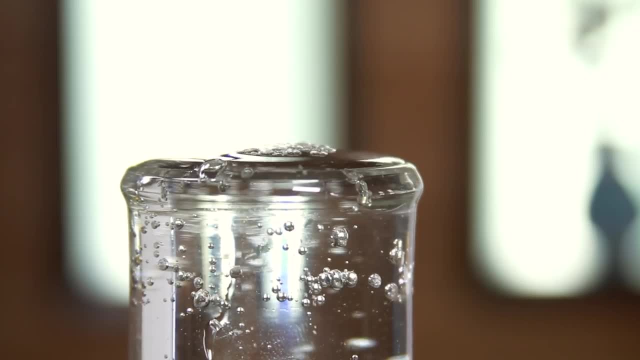 tension depends on the intermolecular forces that pull molecules of a liquid together. These attractive, also called cohesive forces pull the surface molecules inward And what you see when you look at this pile of water is the result of those cohesive forces Minimized. 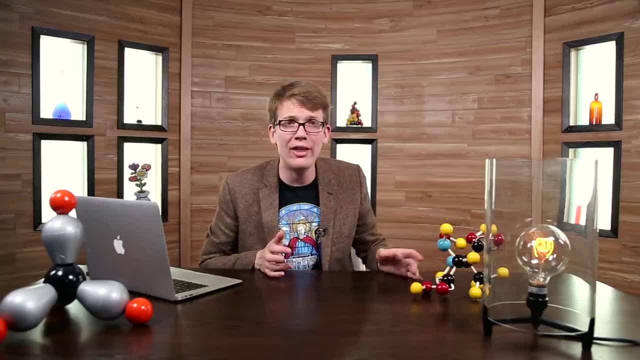 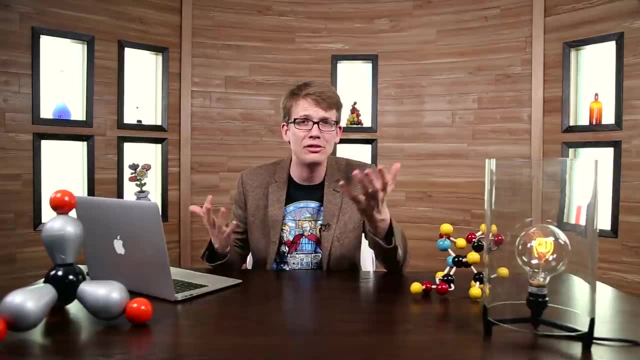 surface area in the water, in this transition water, in this beaker. When you put a bit of oil into that mix, the water totally freaks out. Oils have notoriously non-polar molecules, so suddenly there's this mess of uncharged 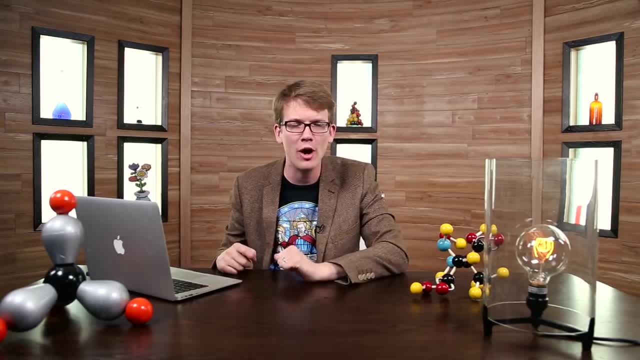 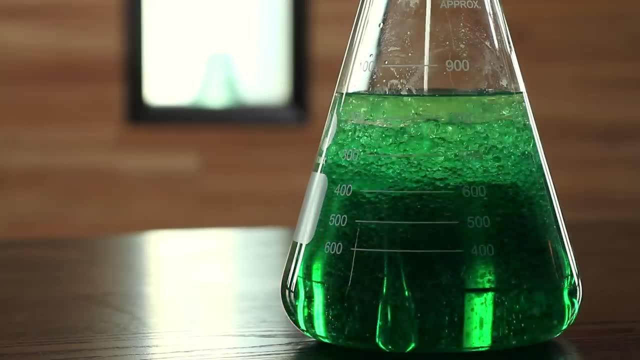 gunk, interfering with the nice orderly arrangement of polar water molecules. But if you take a closer look, the processes are very similar to those between water and air. Water does everything it can to minimize its surface area and kind of expels the oil. 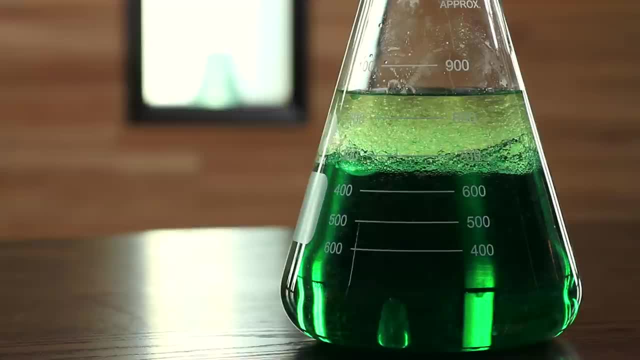 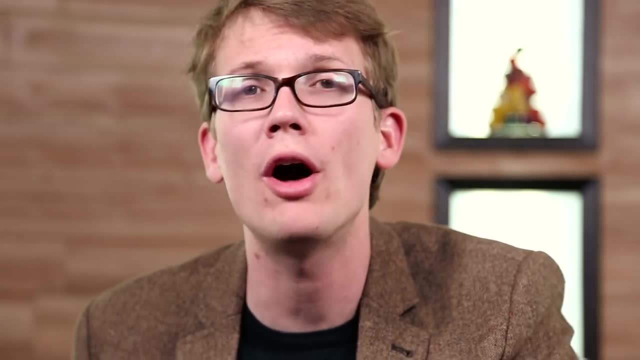 droplets Rather than the water disliking the oil, it actually just likes itself much more, so it won't mix with the oil. Now, if you put polar stuff in water is all about that and those polar water molecules just go after whatever other partial charges they can find. Or, in the case of many ionic 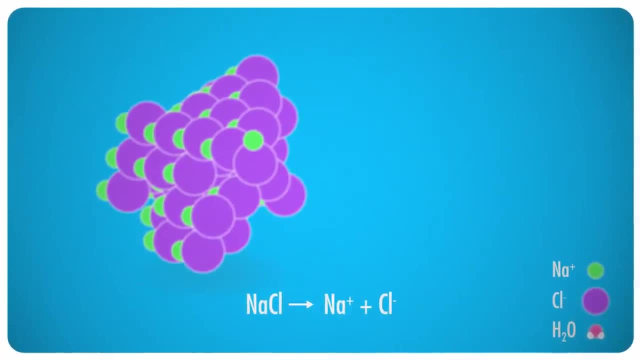 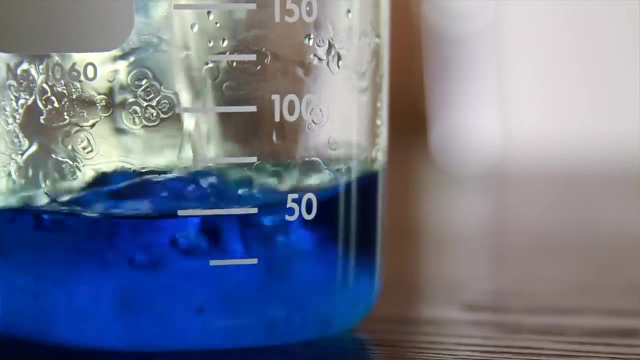 solids. the partial negative charges on the oxygen side all gang up on the positive ions, while the partial positives on the hydrogen side surround the negative ions, breaking the crystals apart and dissolving them into freely moving ions. In some cases, we can actually witness these interactions in unexpected ways. Mix: 50 milliliters. 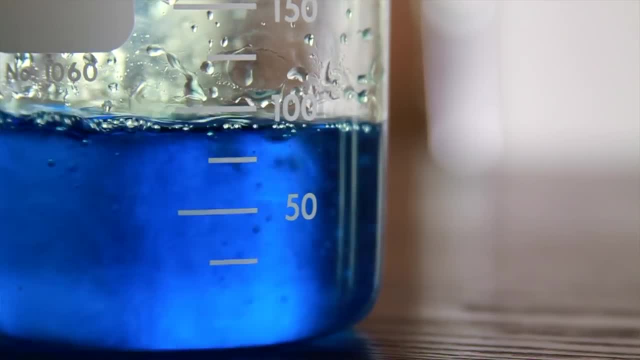 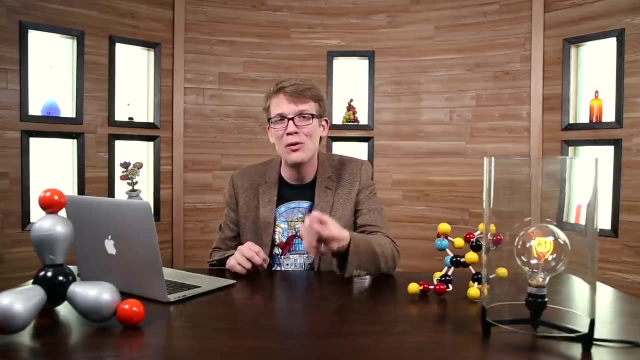 of water with 50 milliliters of water. The polarity of water also results in a phenomenon that makes life possible: Hydrogen bonding. The arrangement of water mixed with alcohol is actually more structured and thus more dense, resulting in a smaller volume. 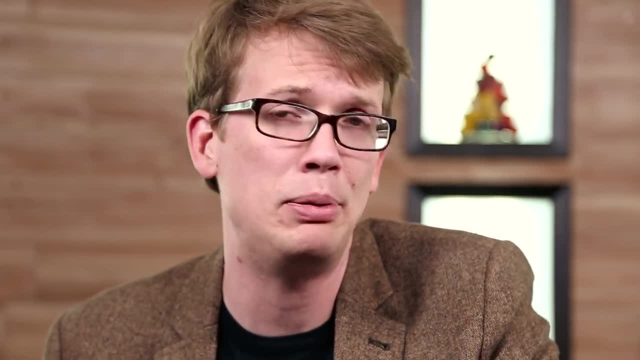 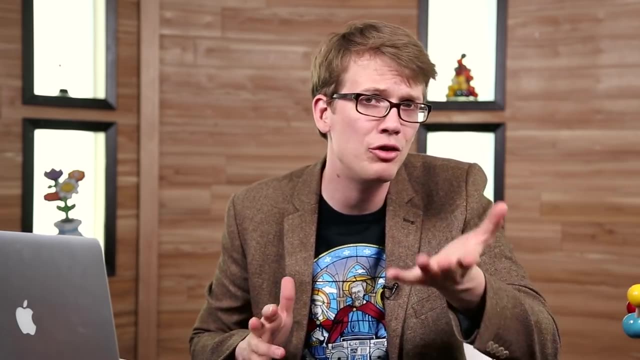 The polarity of water also results in a phenomenon that makes life possible: Hydrogen bonding. The partially negative oxygen and positive hydrogen atoms in a water molecule are not 100% faithful to each other. They engage in additional kind of loose relationships with other neighboring hydrogen and oxygen atoms. 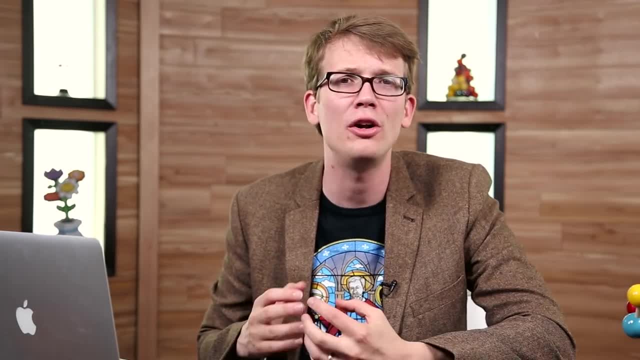 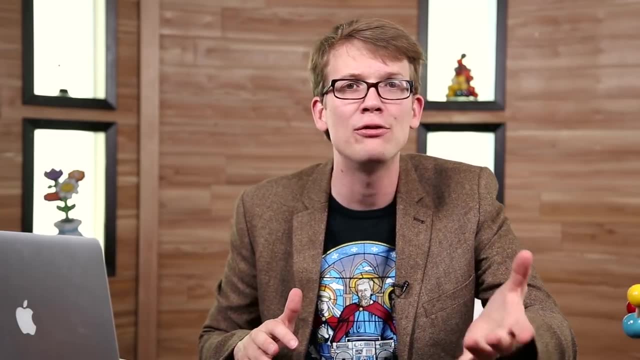 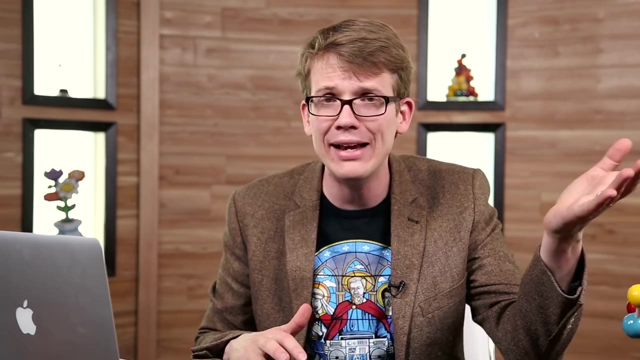 These loose, somewhat fleeting relationships are called hydrogen bonds. In ice, 100% of O and H atoms are involved in hydrogen bonding. The most energetically favorable spatial arrangement of these bonds actually pushes the water molecules apart a bit, resulting in the volume of ice being 10% larger than the volume of water, which 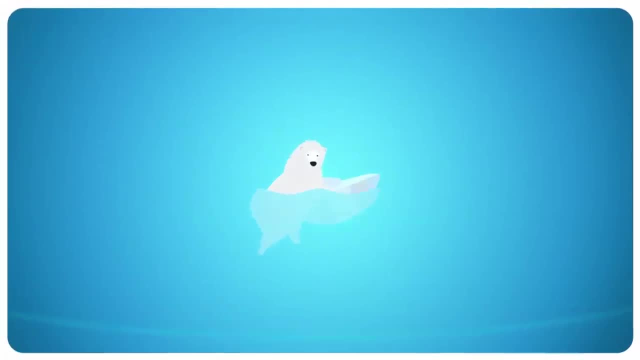 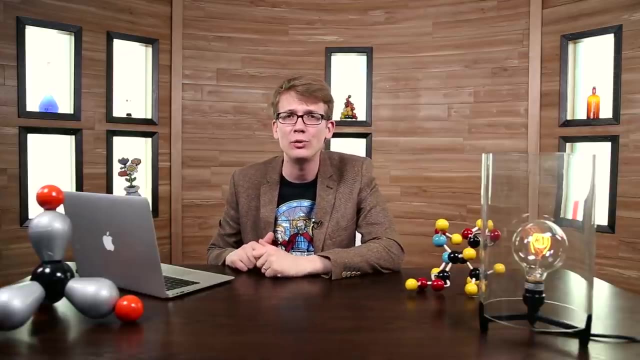 is really weird for solids and liquids. When ice melts, there are still about 80% of Os and Hs engaged in hydrogen bonding, creating ice-like clusters that keep the volume of the cold water relatively high. With rising temperatures, these clusters disappear, while the volume of the truly liquid water rises, resulting in a major characteristic of water having its highest density at 4 degrees Celsius. And yes, that's why ice floats on lakes in the winter and why the bottom of frozen lakes tend to be about 4 degrees Celsius, And also why hockey was invented. 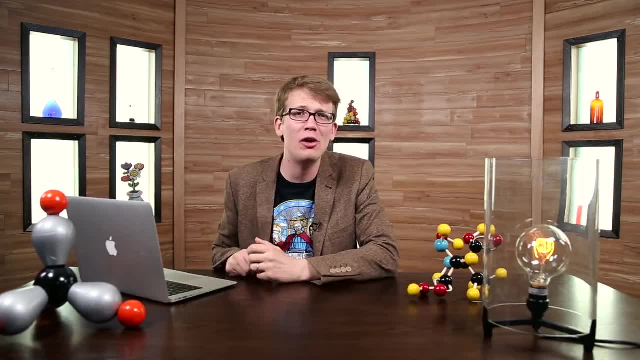 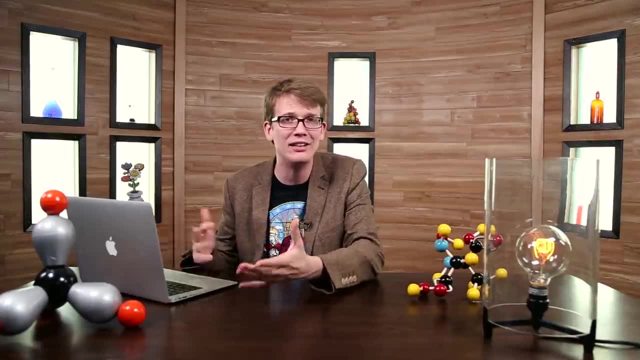 and why soda bottles explode when you leave them in the freezer. But hydrogen bonds are also why taking a warm bath is so great, why steam engines change the world and why temperatures on our planet- Все planet- are so constant when compared to other cosmic temperature fluctuations. 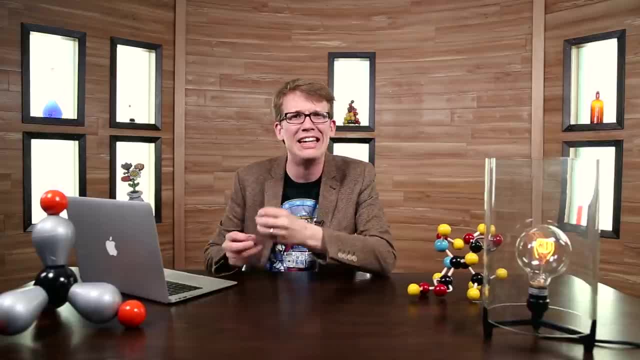 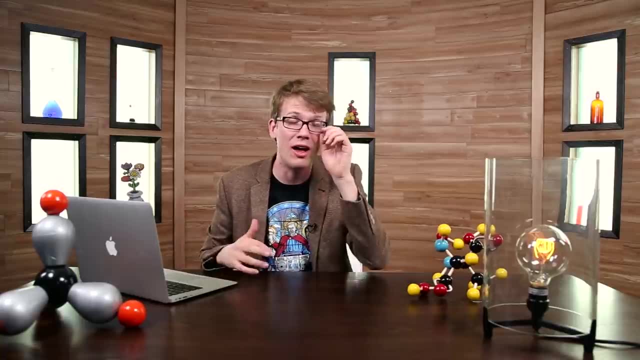 It takes a lot of energy to change the temperature of water, because each little temperature change is associated with breaking or forming lots of hydrogen bonds and they absorb or give off a lot of heat. In fact, the specific heat capacity of water is about five times that of common rocks. 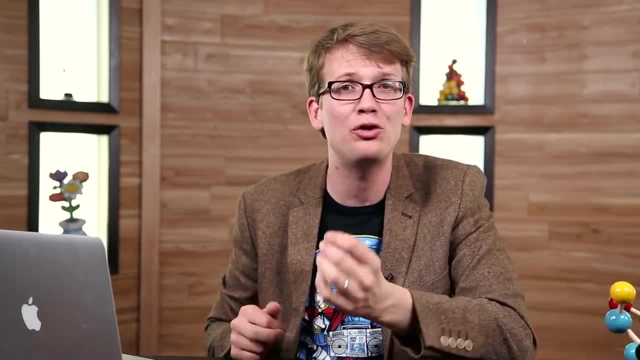 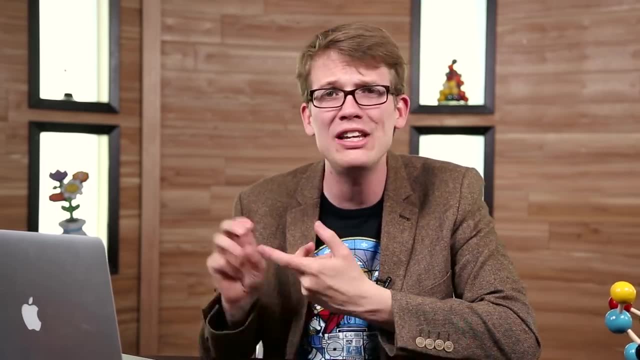 And, amazingly, we haven't even finished talking about how powerfully useful these partial charges are. They also allow water to dissolve pretty much anything that's even partially nonpolar, which includes sugars, proteins, ions and tons of inorganic chemicals.